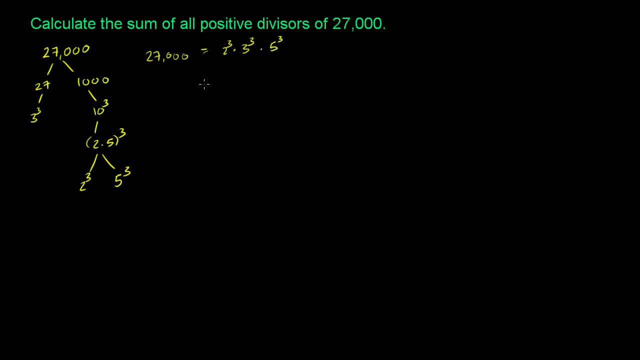 So let's say it has zero 2's. So I'm just going to take the powers of 2's. So if it has zero 2's then we'll put a 1 here. If it has two 2's, then it has to be dissolved by 4.. 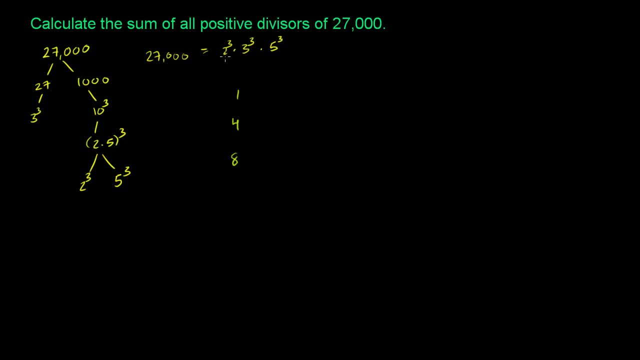 If it has three 2's, it's going to be divisible by 8.. When I say three 2's, I mean 2 times 2 times 2.. Now let's do it with the 3's. Oh wait, I forgot a power. 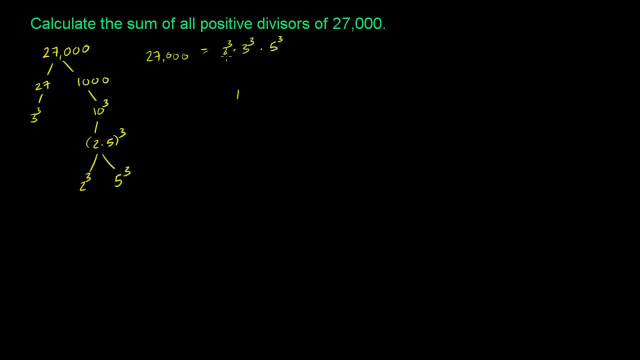 If you have zero 2's, it means it's just divisible by 1, from looking at the 2's, If you have one 2,, it's divisible by just 2.. If you have two 2's, you're divisible by 4.. 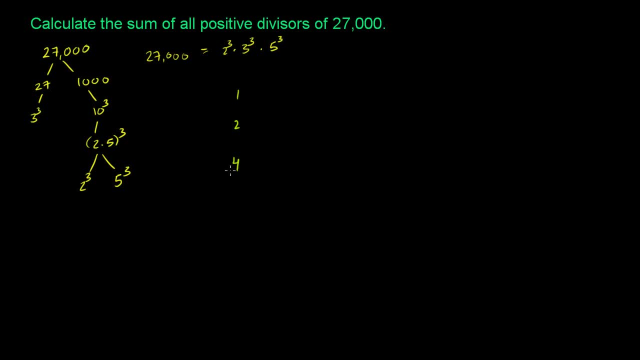 And if you have three 2's- and when I mean that I'm saying 2 times 2 times 2,, that means you're divisible by 8.. Now let's do the same thing with 3.. From the point of view of the 3, if you have no 3's, 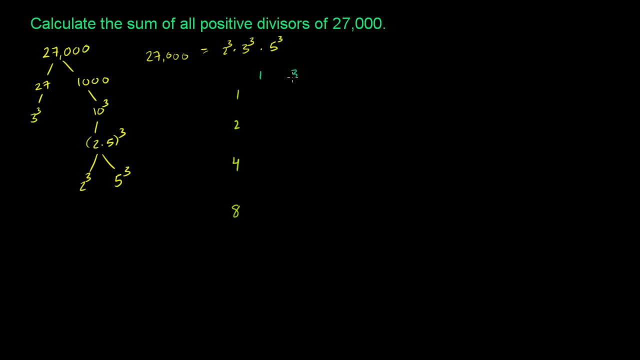 that means at least you're divisible by 1.. If you have one 3,, that means you're divisible by 3.. Two 3's or 3 times a 3, means you're divisible by 9.. If you have three 3's, it means you're divisible by 27.. 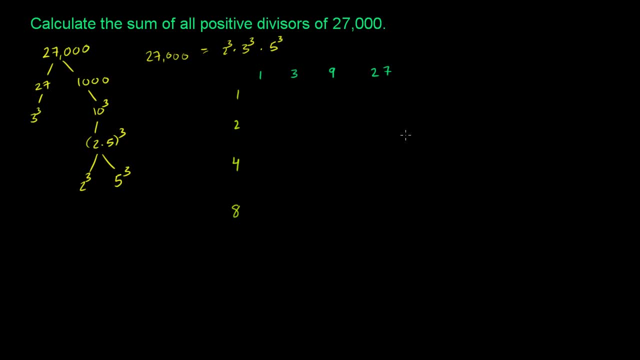 So let's look at all of the possible combinations And for this grid that I'm going to generate right here, we assume that you're not divisible by 5, or you're only divisible by 5 to the 0 power. So what are all the possible numbers here? 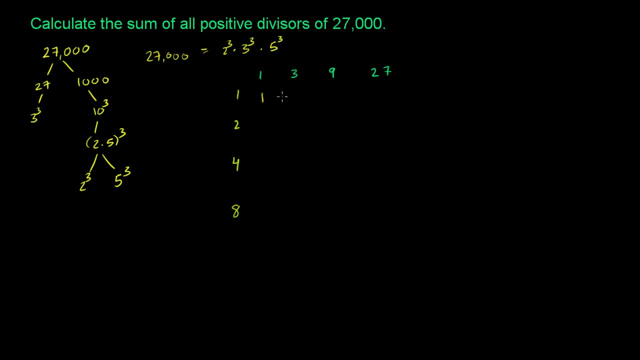 Well, you have 1 times 1.. That's divisible by 1 and 1.. You have 1 times 3,, which is 3.. 1 times 9,, which is 9.. 1 times 27,, which is 27.. 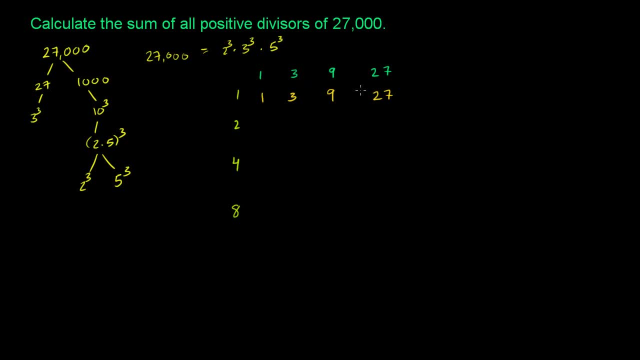 So these are all the numbers that have up to three 3's in them, from 0 to three 3's in them, And they have no 2's in them. If you throw another 2 in here, you're essentially going to multiply all of these numbers by 2.. 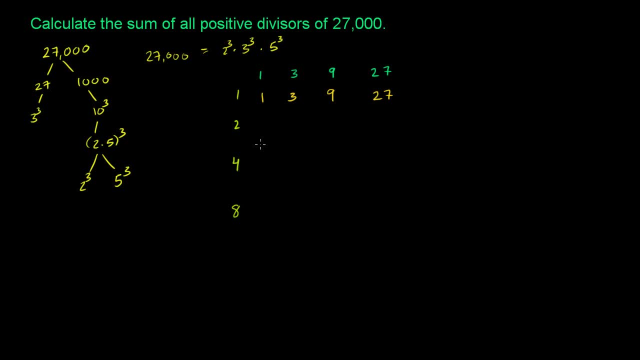 If you throw another 2 in here, you're going to multiply all of these numbers by 2.. Now, before I do this- because I want to do this as fast as possible- I could figure out what these numbers are. I could multiply them. 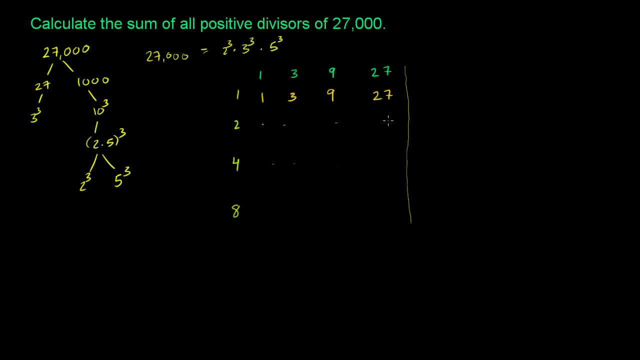 But instead, let's just take the sum. Let's just take the sum here of this row, of this first row that we just did. We have 1 plus 3 plus 9 plus 27.. 3 plus 27 is 30.. 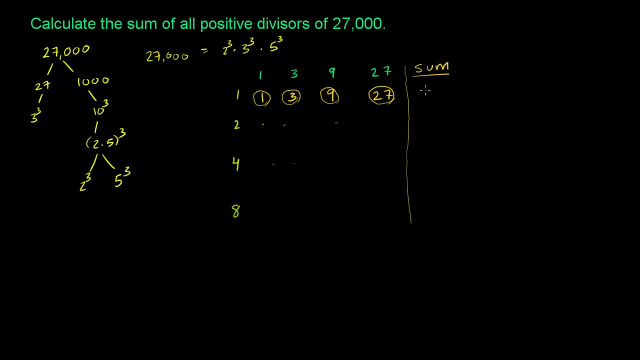 1 plus 9 is 10.. So this is going to be 40.. Now, whatever these numbers are, they're all going to be 2 times these numbers. So the sum is going to be 80.. And the sum over here is going to be 2 times the previous row. 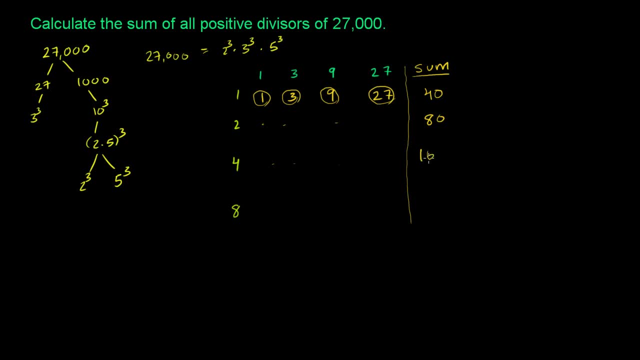 because here we multiplied by 2.. Here we're multiplying by 4. So it's going to be 160. And over here we just multiply by 2, again It's going to be 320. Or another way of thinking about it. whatever the sum is here. 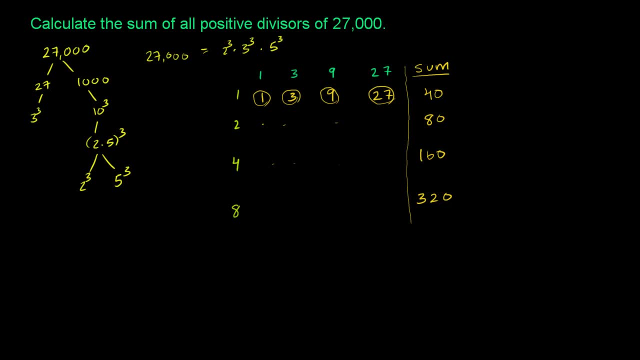 it's going to be 8 times the sum of the first row And just so you know what I'm doing, I could actually put numbers here. This number here would be 8,, 24,, 72, and whatever. 8 times 27. 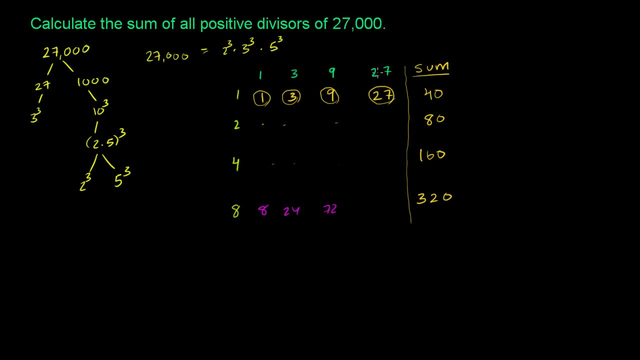 had with that 160.. 160 plus 56, so it's 216.. But we don't want to do that, We just have to think about the sums. So if you think about all of the divisors of 27,000. 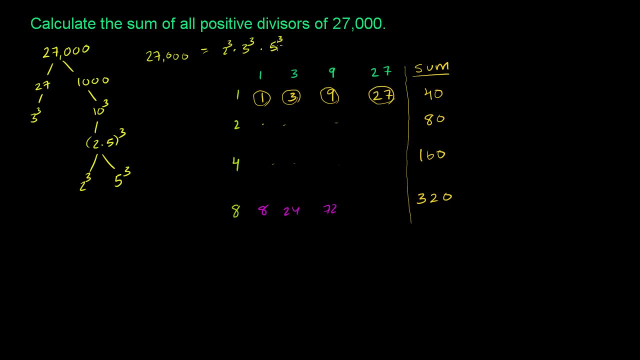 that are not divisible by 5, so they're only divisible by 5 to the 0-th power. I guess you could say it. we have now figured out their sum. It's going to be the sum of all of these rows. 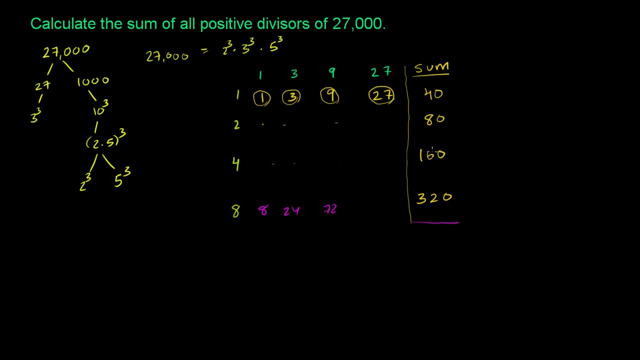 So if you take 40 plus 80,, you have 120.. Plus 160 is 280.. Plus 320 is 600.. So this is the situation. This is the sum of all of the combinations of the 2's and the 3's that don't have any 5's in them. 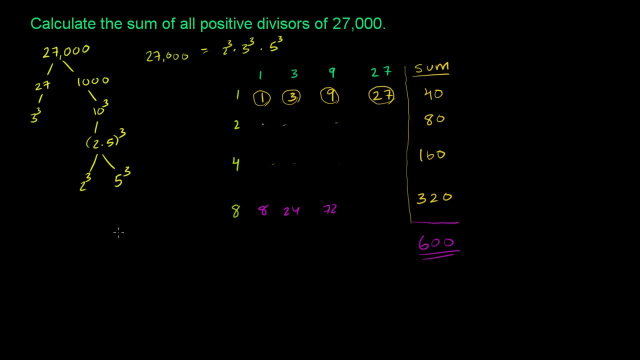 Now, if you took the same combination of 2's and 3's, so these added up to 600.. Let me write it over here: These added up to 600.. So no 5's Now if you did the same exact thing that we just did here. 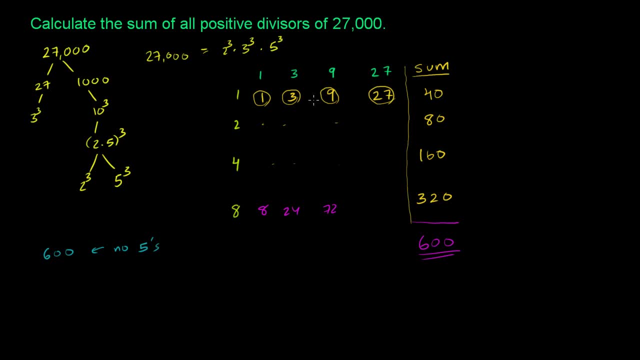 but we just multiplied everything by 5.. So we'd then be looking at all the combinations that have this many 2's and this many 3's and one 5.. OK, So if you did the same exact thing that we just did here, 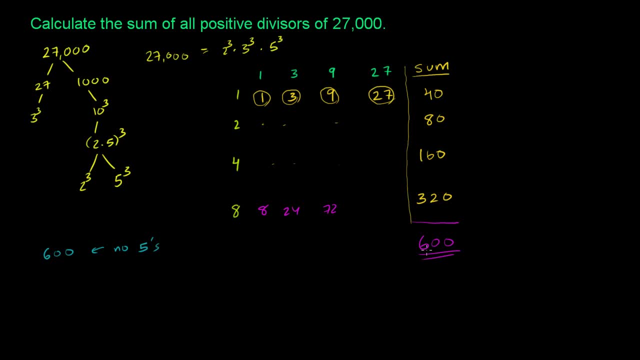 we'd then be looking at all the combinations that have this many 2's and this many 3's and one 5.. What would happen to this sum? Well, we would just multiply it by 5.. So let's multiply that by 5.. 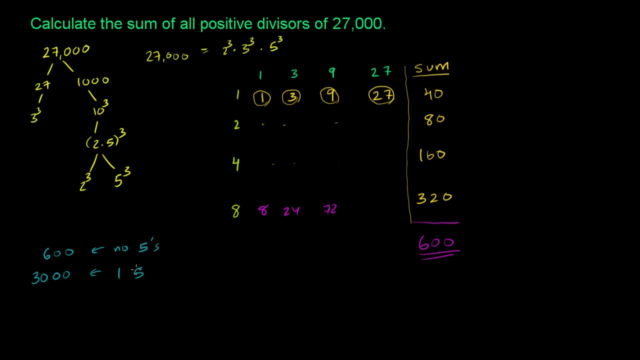 So you multiply 600 by 5, you get 30 with two 0's, And so this is 1, 5 in the prime factorization of the divisors 1,, 1, 5.. Just like that. 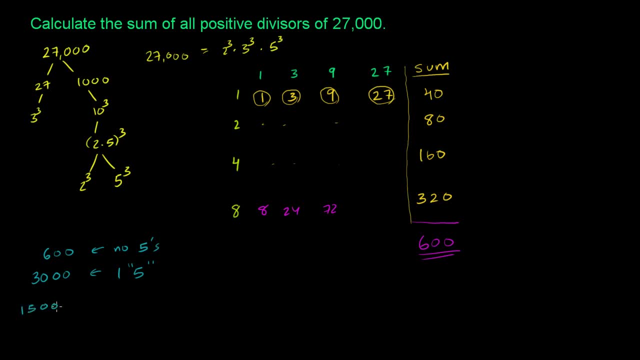 Now, if I wanted 2- 5's, I could just multiply by 5 again. So if I multiply by 5 again, I get 15.. 15,000.. This is 2- 5's- Another way of thinking about this. 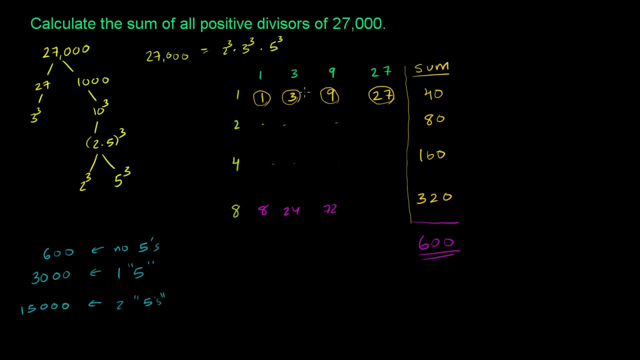 if I just multiply this whole, every term here, by 25,, which is essentially multiplying by 5 times 5,, this sum is going to be 600 times 25,, which is 15,000.. Now if I have 3 5's, then I could just multiply this by 5 again. 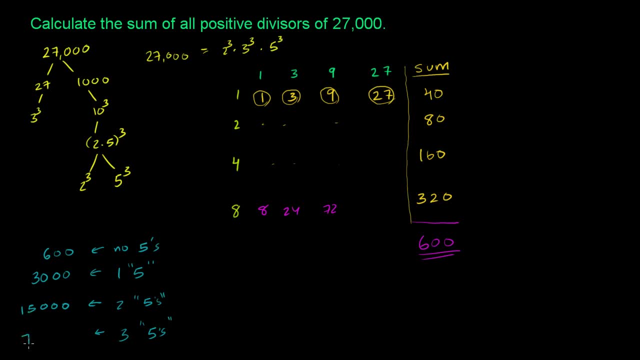 5 times 15 is 15 plus 25 is 7.. So it's 75,000.. So now I know all the sums. If I have no 5's, the sum of all the divisors is 600.. I have 1, 5,, 3,000, so on and so forth. 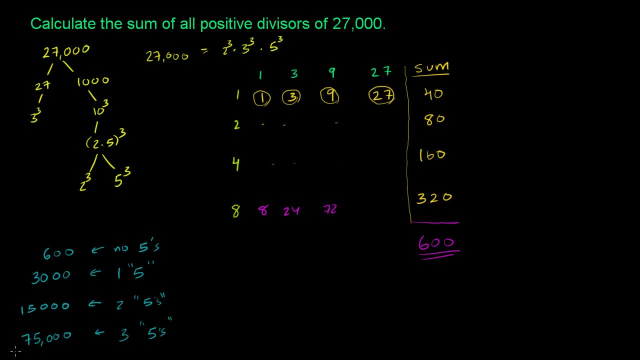 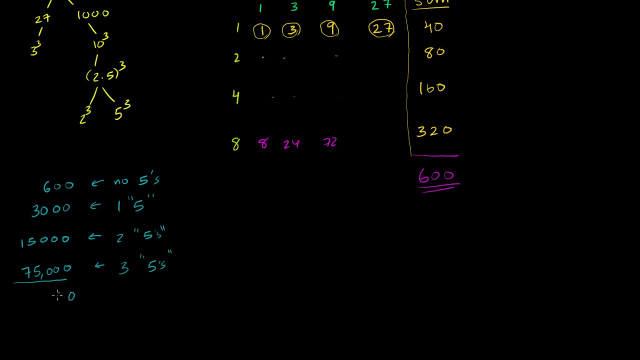 So if I want the sum of everything, I just take the sum of these numbers. Let me scroll down a little bit So I get. well, I have 0,, 0. Then in the 100's place I only have a 6.. 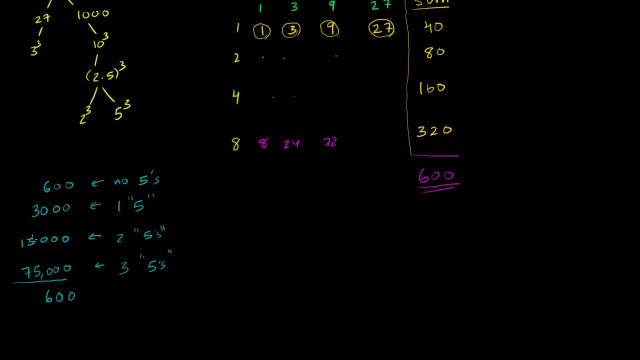 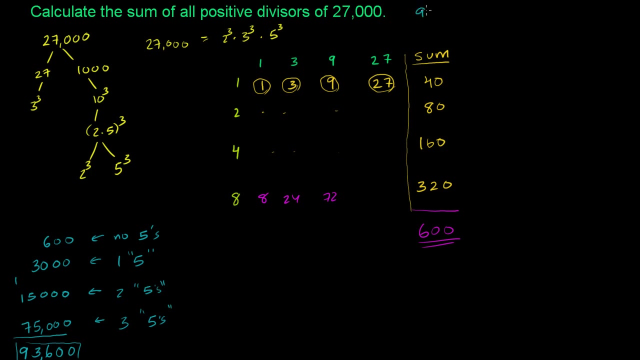 And then 3 plus 5 plus 5 is 13.. Is that right? Yep, that's 13.. And then carry the 1,, and then I have a 9.. So I have 93,600.. So the sum of all positive divisors of 27,000, 93,600.